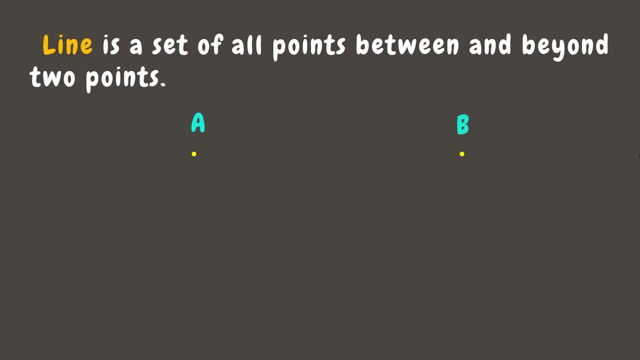 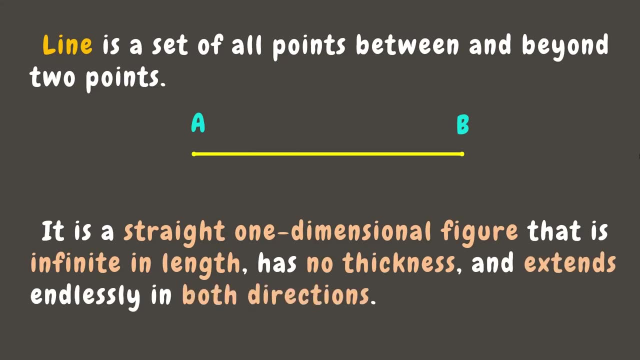 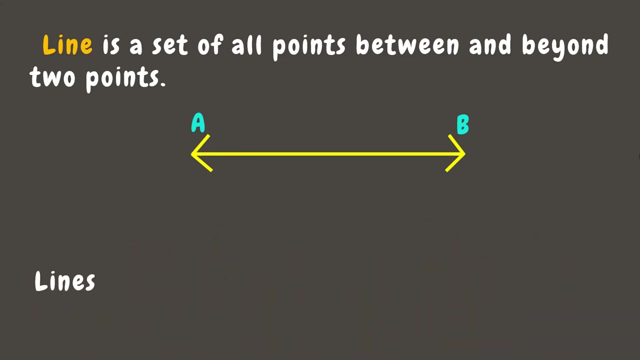 If we connect the two points, it will create a line. A line is a one-dimensional figure that is infinite in length, has no thickness and extends endlessly in both directions. Lines can be named using two points on the line. Since this line has point A and point B, it can be called as line AB. 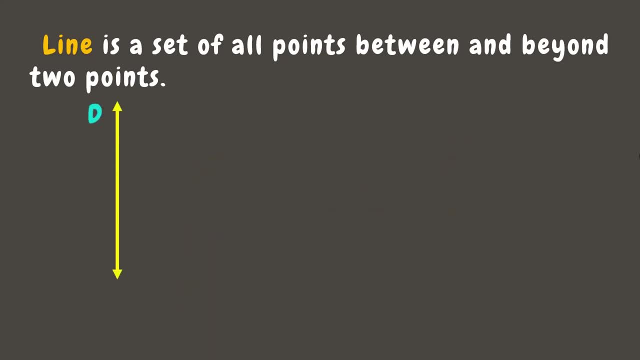 A line that goes from top to bottom is called vertical line. This means that line DE is a vertical line. A line that goes from right to left is a horizontal line. This means that line XY is horizontal, While this kind of line is a diagonal line. 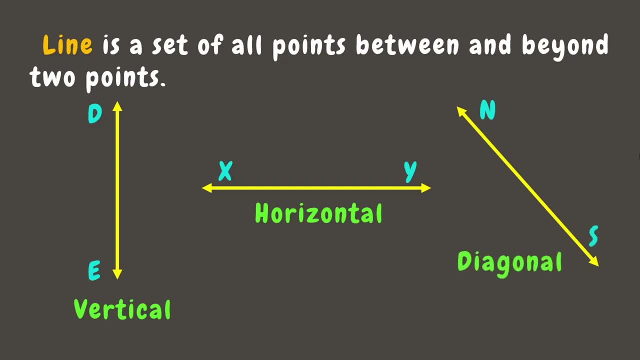 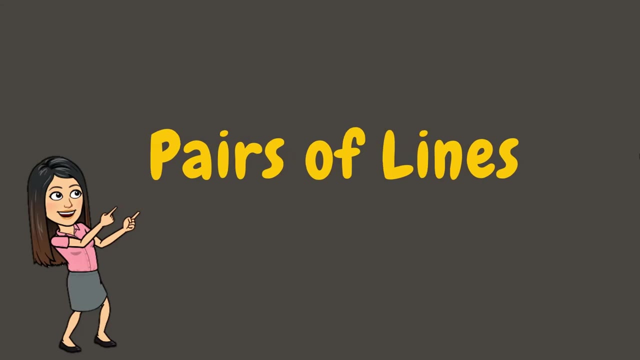 This means that line NS is diagonal. These are only a few of the many kinds of lines. There are other kinds of lines that are also called as pairs of lines. What are those? Let's find out. First. we have parallel lines. 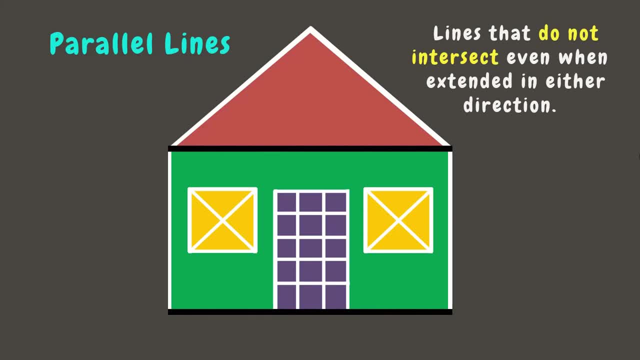 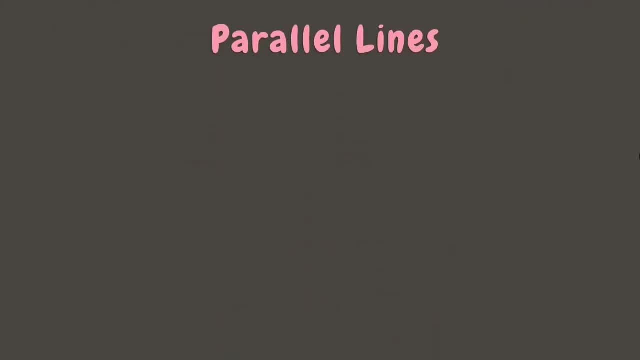 These are the lines that do not intersect or cross each other, even when extended in either direction. Parallel lines can be a pair of vertical lines, Vertical lines, A pair of horizontal lines Or a pair of diagonal lines, As long as they don't intersect or cross toward each other. 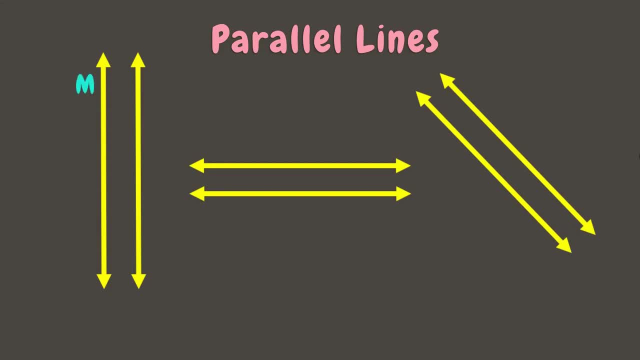 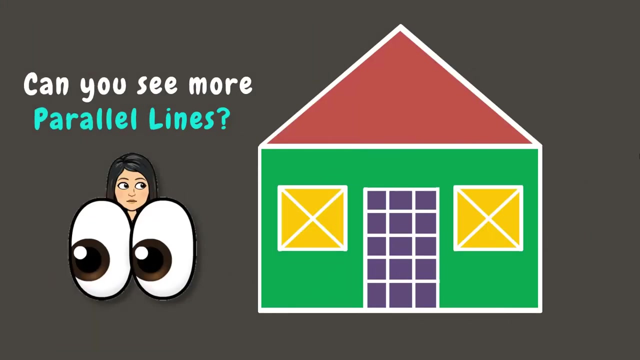 So here we can say that lines MK and line SB are parallel, Same with line LO and line GH. they are parallel, And line JF and PW are parallel. Let's go back to our drawing. Can you see more parallel lines? 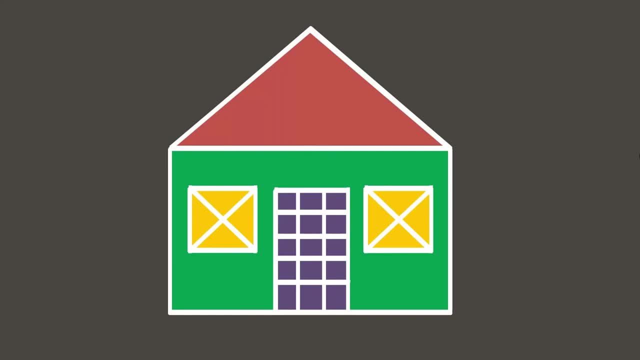 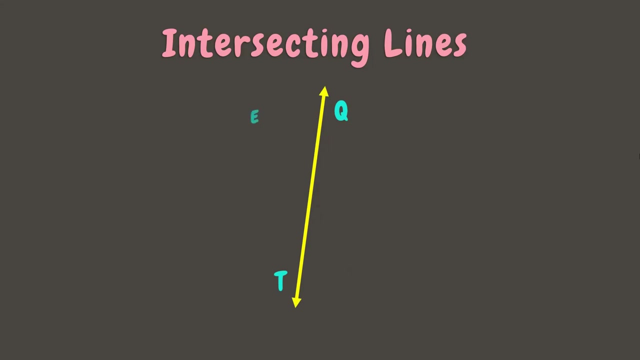 Now let's go to the next one. Next pair of lines is what we call intersecting lines. Unlike parallel lines, these lines meet or intersect at a certain point, even when extended Here. in another example we can see that line QD and line ER cross each other at a certain point. 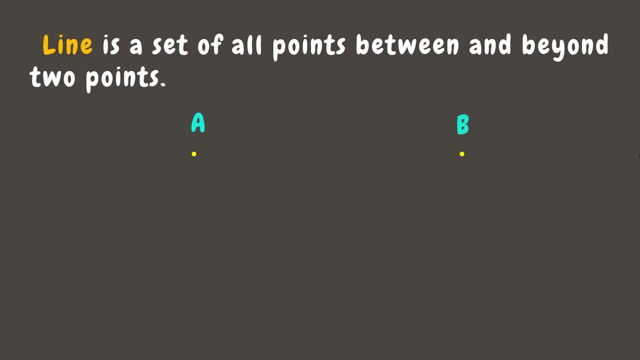 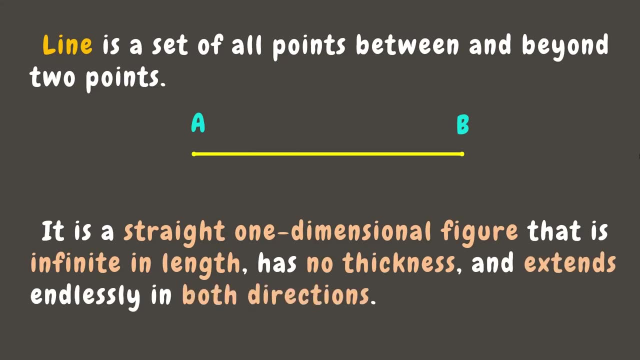 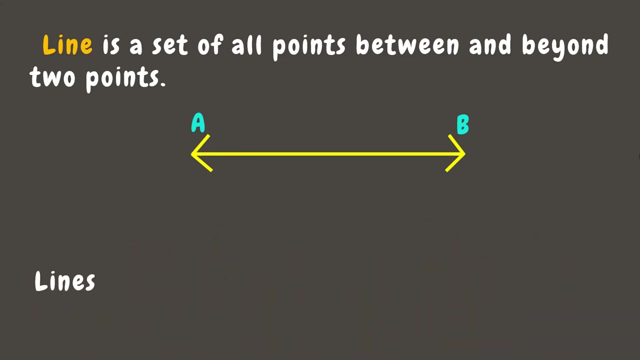 If we connect the two points, it will create a line. A line is a one-dimensional figure that is infinite in length, has no thickness and extends endlessly in both directions. Lines can be named using two points on the line. Since this line has point A and point B, it can be called as line AB. 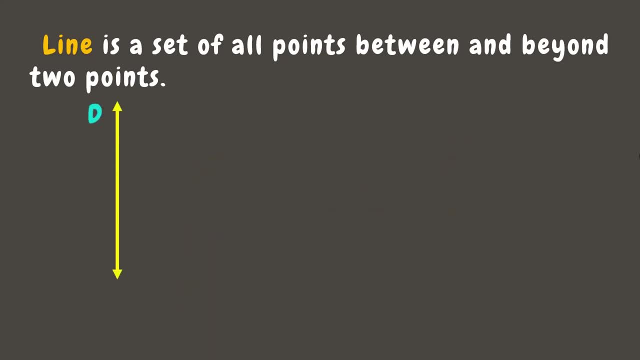 A line that goes from top to bottom is called vertical line. This means that line DE is a vertical line. A line that goes from right to left is a horizontal line. This means that line XY is horizontal, While this kind of line is a diagonal line. 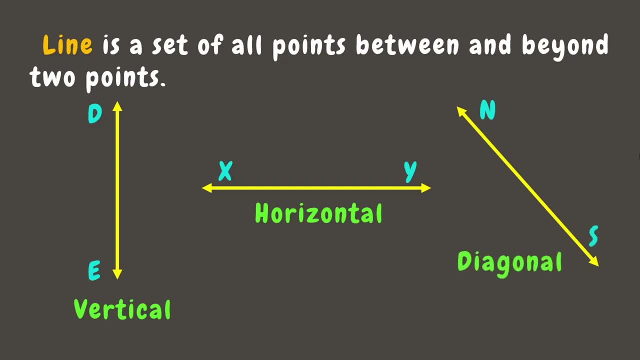 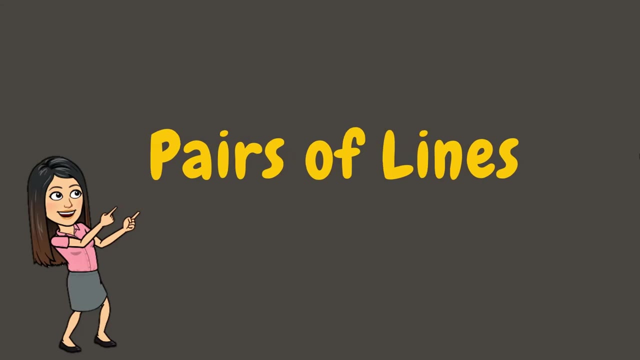 This means that line NS is diagonal. These are only a few of the many kinds of lines. There are other kinds of lines that are also called as pairs of lines. What are those? Let's find out. First. we have parallel lines. 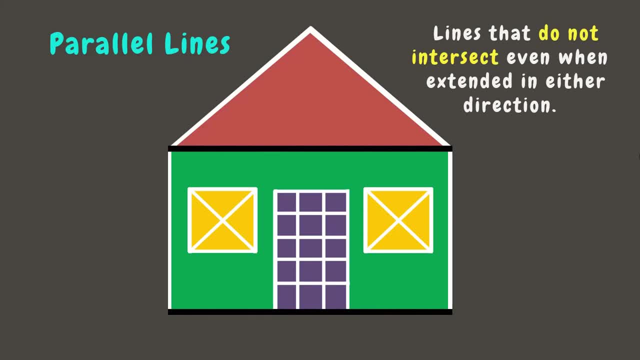 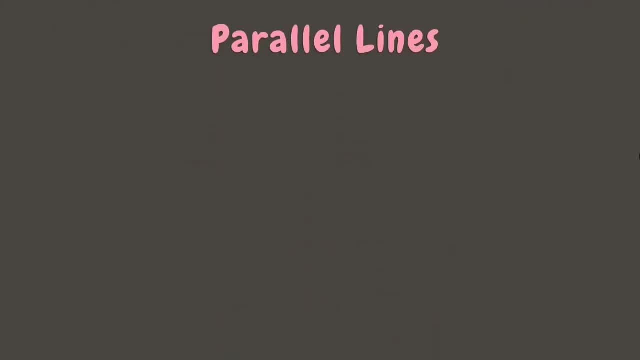 These are the lines that do not intersect or cross each other, even when extended in either direction. Parallel lines can be a pair of vertical lines, Vertical lines, A pair of horizontal lines Or a pair of diagonal lines, As long as they don't intersect or cross toward each other. 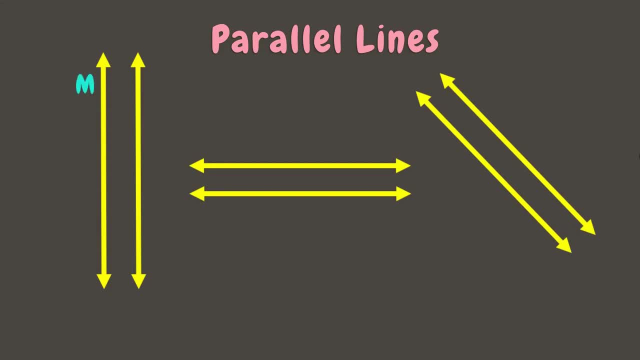 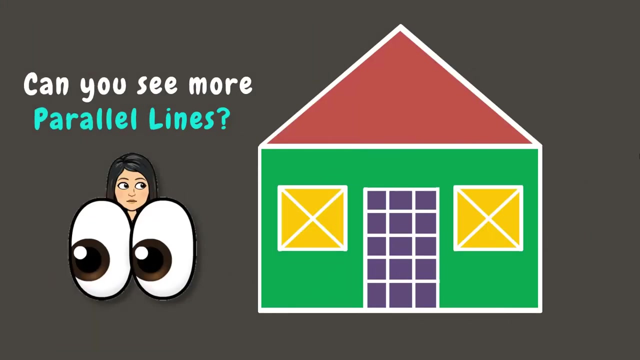 So here we can say that lines MK and line SB are parallel, Same with line LO and line GH. they are parallel, And line JF and PW are parallel. Let's go back to our drawing. Can you see more parallel lines? 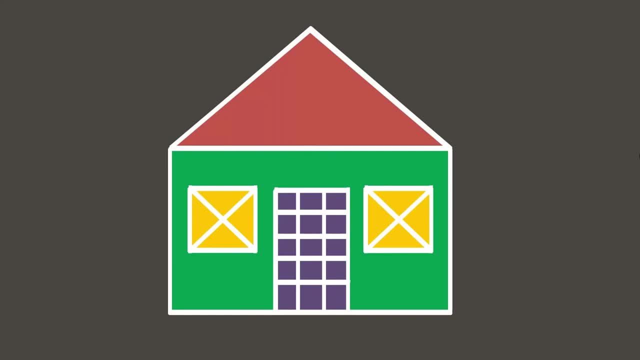 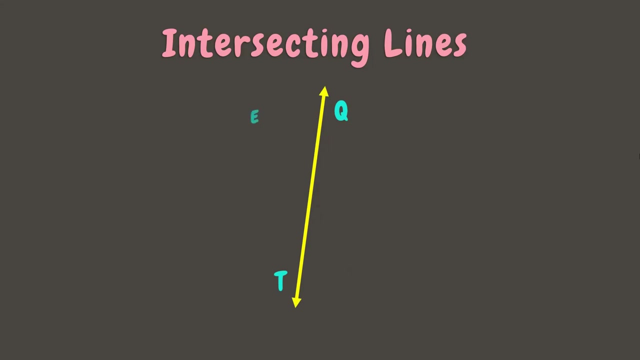 Now let's go to the next one. Next pair of lines is what we call intersecting lines. Unlike parallel lines, these lines meet or intersect at a certain point, even when extended Here. in another example we can see that line QD and line ER cross each other at a certain point. 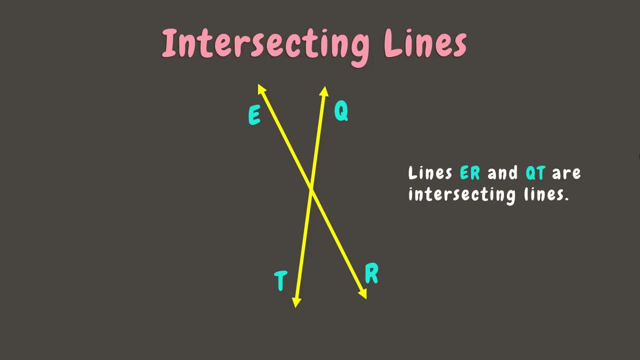 It means that they are a pair of intersecting lines, Same with vertical lines. They meet or intersect at a certain point. This is where lines meet is called point of intersection. For example, here, point B is the point of intersection. Now let's go back to our drawing. 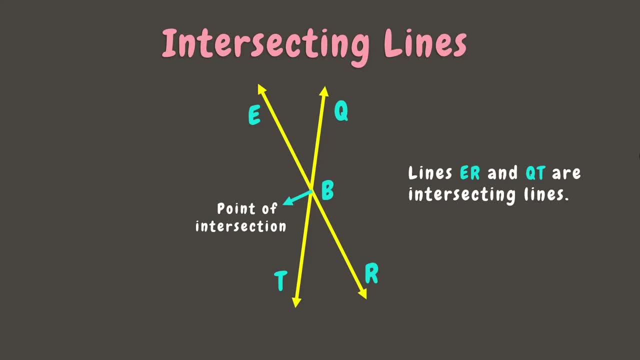 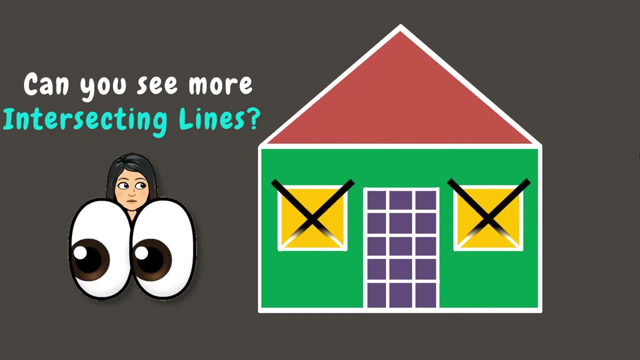 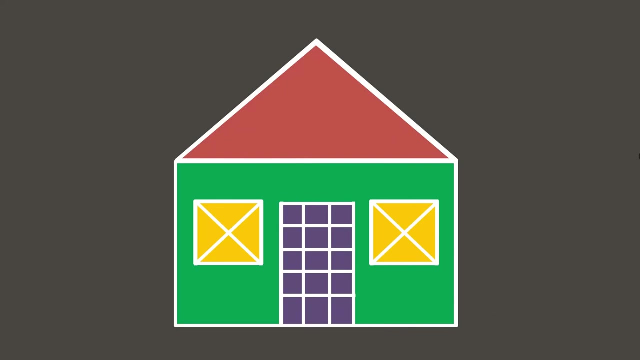 Can you see more intersecting lines? Lastly, we have perpendicular lines, Same as intersecting lines. perpendicular lines are lines that intersect because they are parallel And perpendicular lines are lines that intersect after they intersect. they are parallel, Same as intersection lines. perpendicular lines are lines that intersect. 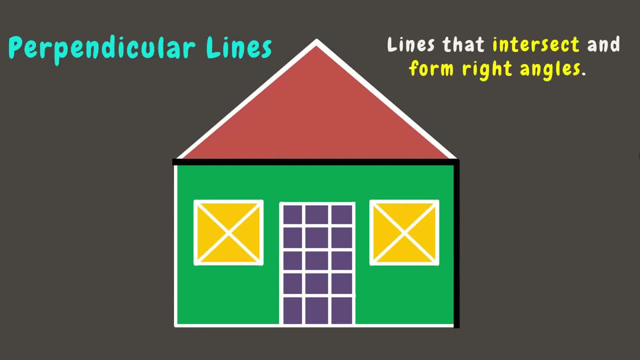 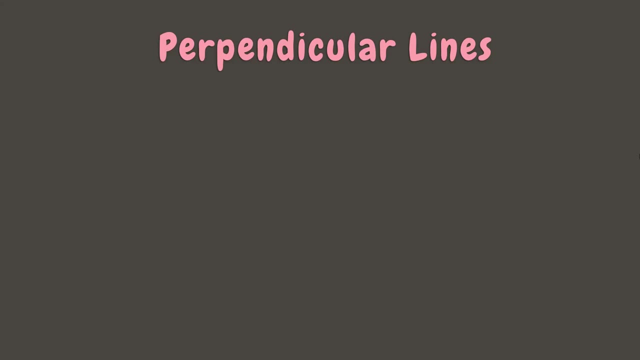 So these are lines that intersect. You can see that now- let's make some drawing- intersect, but the only difference is that they form a right angle as they cross each other. Usually, lines that intersect and form a right angle is a pair of a vertical and horizontal. 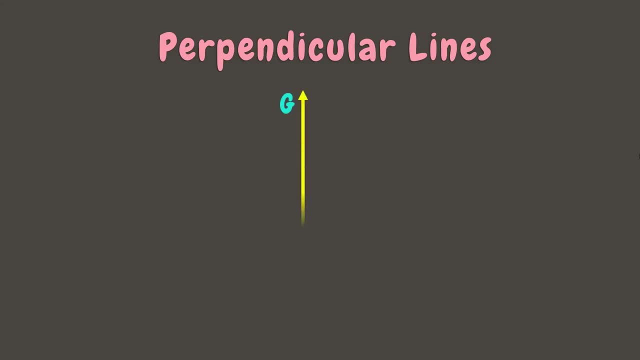 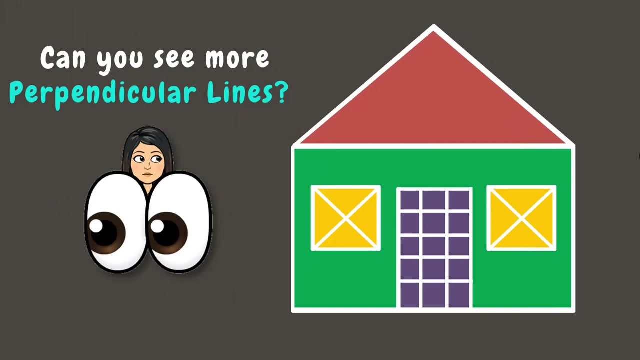 line. Let's say we have vertical line GH which is intersected by horizontal line SB. If two intersecting lines form a right angle like this, therefore, lines GH and SB is a pair of perpendicular lines. Now can you see more perpendicular lines in this drawing? 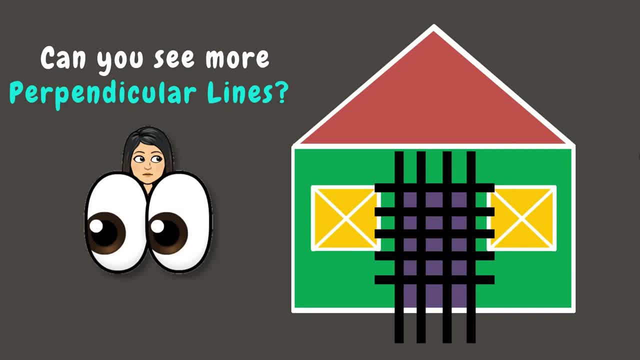 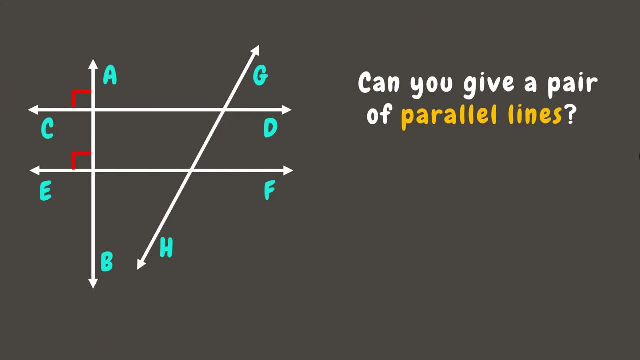 Wonderful. now let's try this activity. Can you give a pair of parallel lines? from the line shown Here we can see that line CD and EF are parallel lines, since they don't intersect or cross each other. Next one: Can you give pairs of intersecting lines? 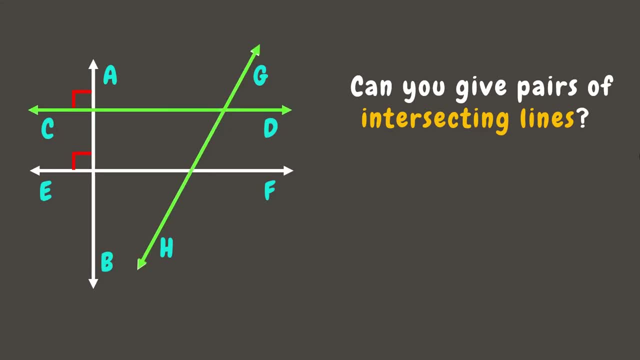 Here we can see that line CD and EF are parallel lines, since they don't intersect or cross each other. Here we can see that lines GH and CD are intersecting lines. Also, lines GH and EF intersect each other, so they are intersecting lines. 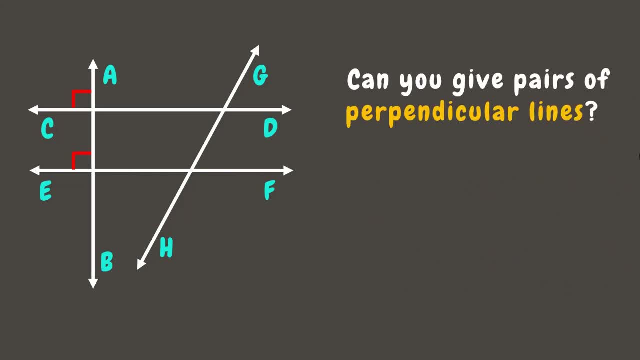 Last one: Can you give pairs of perpendicular lines? We can see that lines AB and CD intersect each other and form a right angle. It means that they are perpendicular lines. Also, lines AB and EF form a right angle as they intersect. Therefore they are also perpendicular lines. 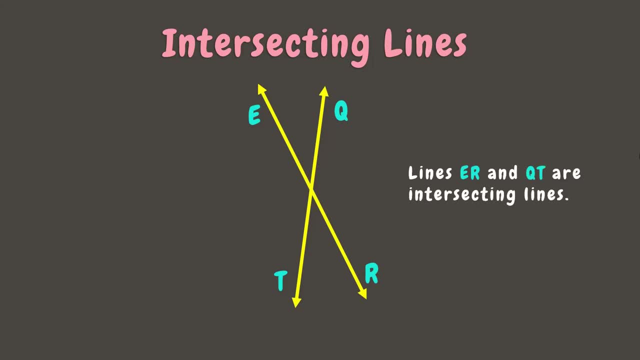 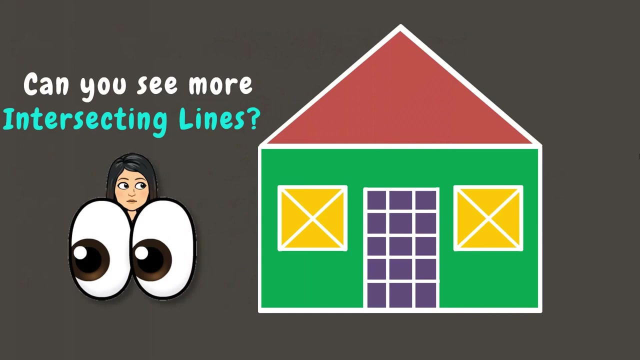 It means that they are a pair of intersecting lines. Our lines meet is called point of intersection. For example, here, point B is the point of intersection. Now let's go back to our drawing. Can you see more intersecting lines? Lastly, we have perpendicular lines. 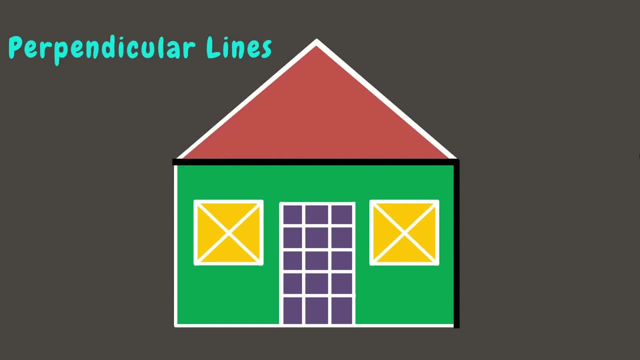 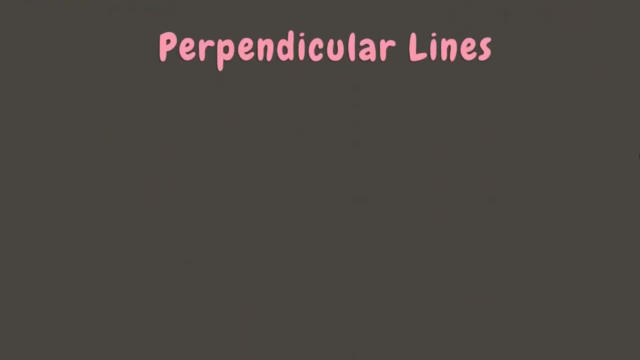 Same as intersecting lines. Perpendicular lines are lines that intersect, but the only difference is that they form a right angle as they cross each other. Usually, lines that intersect and form a right angle is a pair of a vertical and horizontal line. Let's say we have vertical line GH, which is intersected by horizontal line SB. 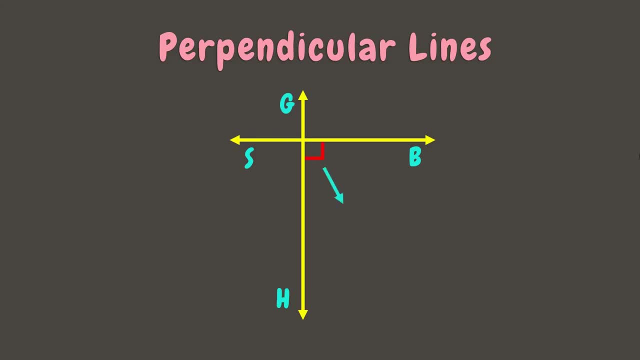 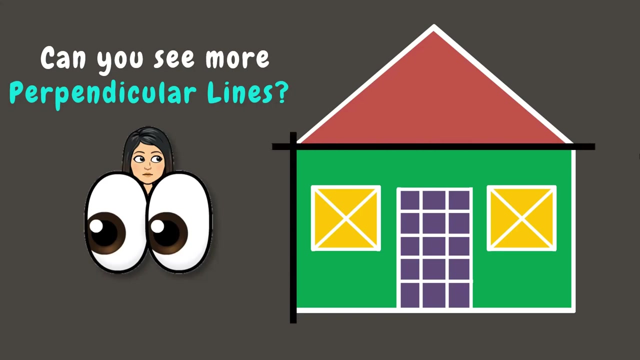 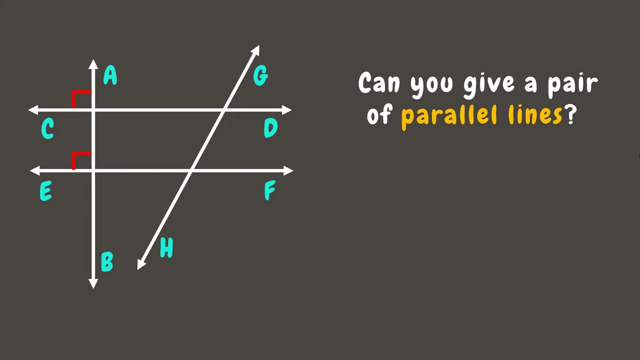 If two intersecting lines form a right angle like this. therefore, lines GH and SB is a pair of perpendicular lines. Now can you see more perpendicular lines in this drawing? Wonderful, now let's try this activity. Can you give a pair of parallel lines from the line shown? 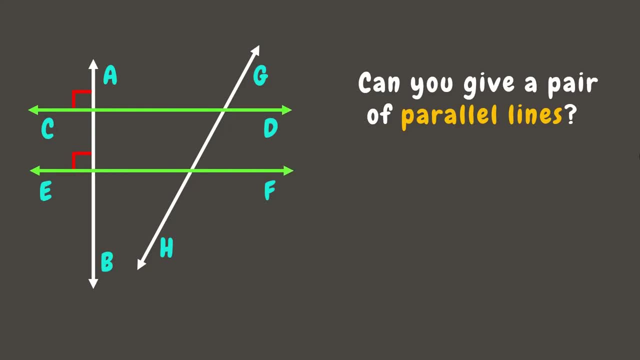 Here we can see that line CD and EF are parallel lines, since they don't intersect or cross each other. Next one: can you give pairs of intersecting lines? Here we can see that line CD and EF are parallel lines, since they don't intersect or cross. 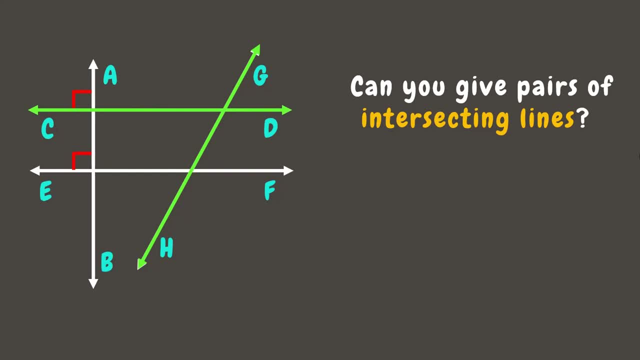 each other. Here we can see that line GH and CD are intersecting lines. Also, lines GH and EF intersect each other, so they are intersecting lines. Last one: can you give pairs of perpendicular lines? We can see that lines AB and CD intersect each other and form a right angle.